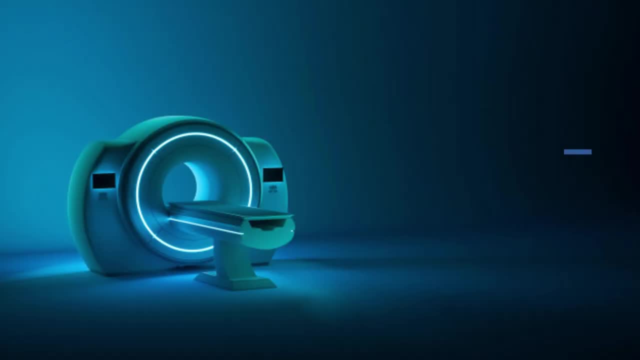 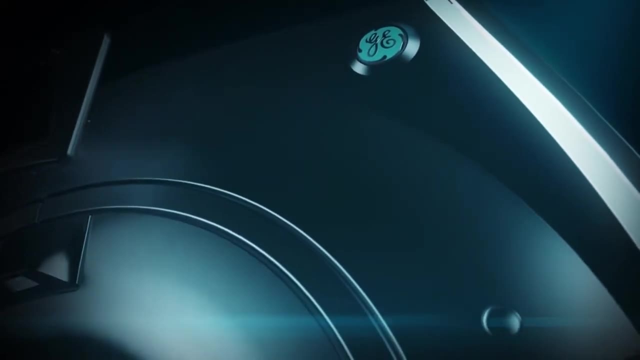 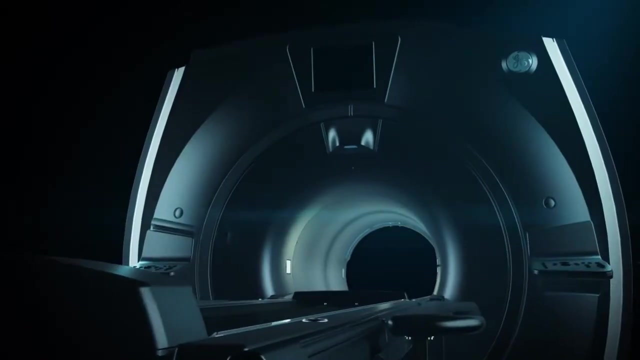 first Let's begin with the components of MRI machines. The major components of an MRI scanner are the main magnet which polarizes the sample, the shim coils for correcting the homogeneities in the main magnetic field, the gradient system which is used to localize the MR signal, and the 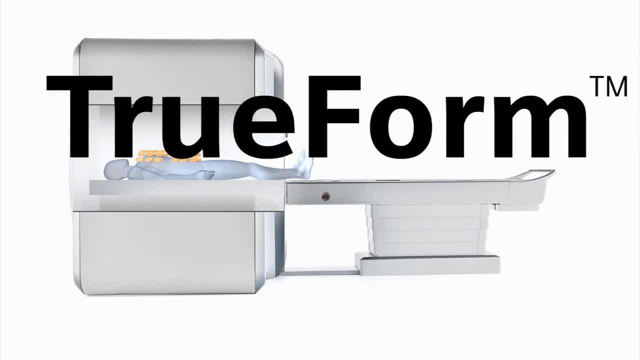 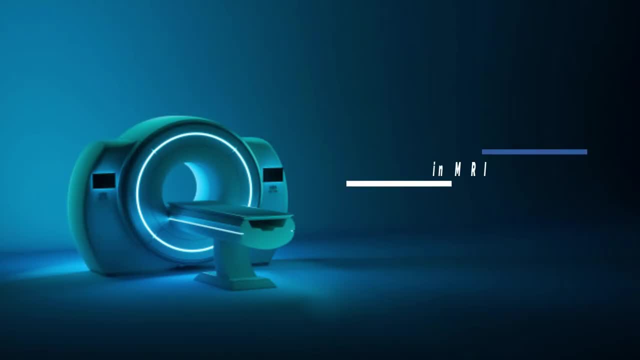 RF system which excites the sample and detects the resulting NMR signal. The whole system is controlled by one or more computers. The first component of the MRI scanner is the magnet in the MRI machine. The magnet is the largest and most expensive component of the 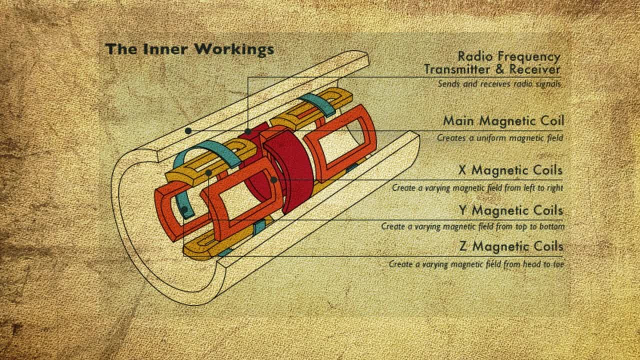 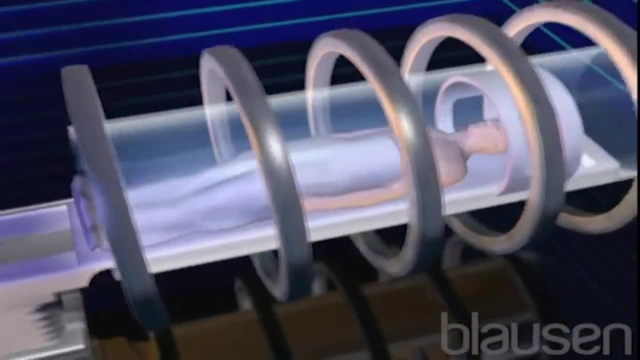 scanner and the remainder of the scanner is built around it. The strength of the magnet is measured in teslas or T. Clinical magnets generally have a field strength in the range of 0.1 to 3.0 T, with research systems available up to 9.4 T for human use and 21 T for animal systems. 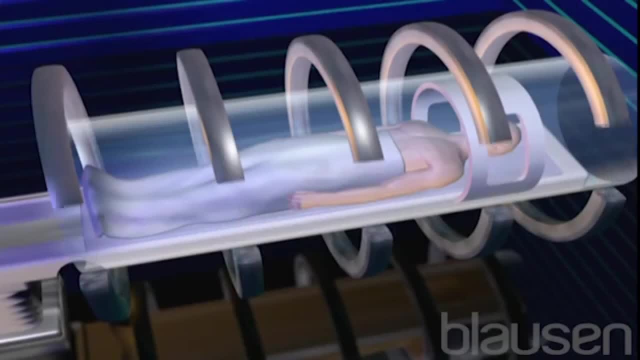 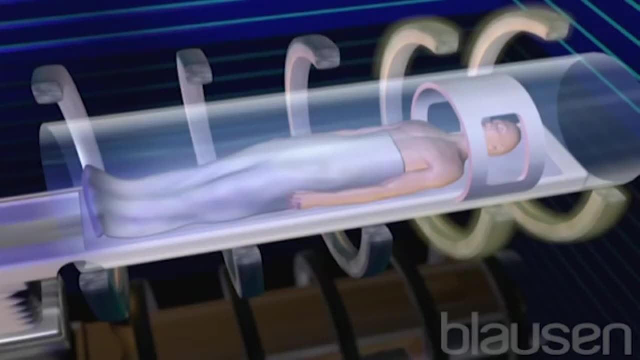 In the United States, field strengths up to 4 T have been approved by the United States Department of Health and Human Services. The United States Department of Health and Human Services has been approved by the FDA for clinical use. There are different types of magnetic principles which are used, like permanent magnet, resistive electromagnet and superconducting. 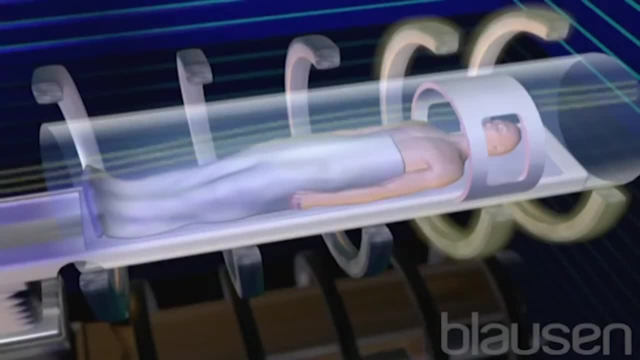 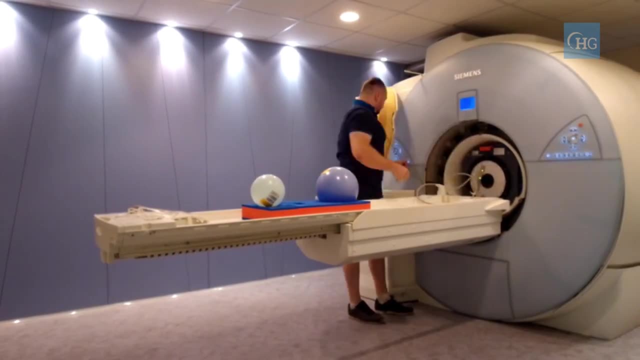 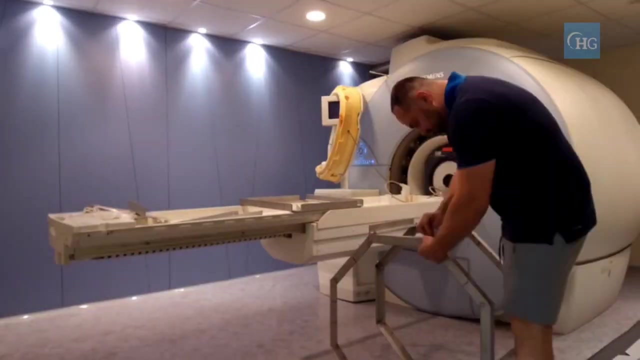 electromagnet. The second component is shims in the MRI machine. When the MR scanner is placed in the hospital or clinic, its main magnetic field is far from being homogeneous enough to be used for scanning. That is why, before doing fine-tuning of the field using a sample, the magnetic field of 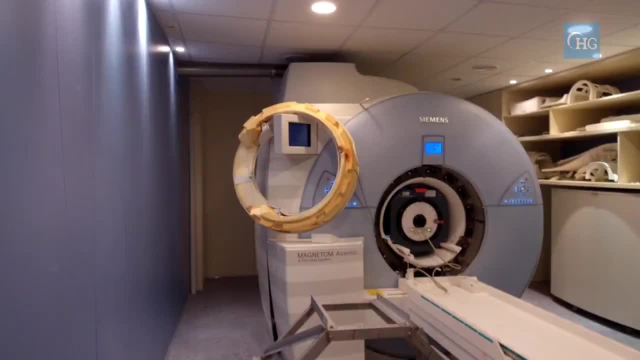 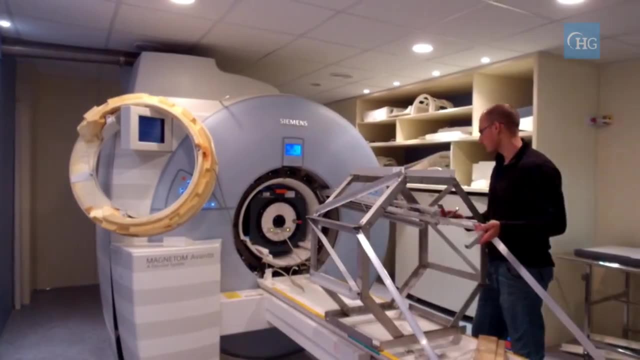 the magnet must be measured in order to be able to measure the magnetic field of the MRI machine. After a sample is placed into the scanner, the main magnetic field is distorted by susceptibility boundaries within that sample, causing signal dropout, regions showing no signal and spatial 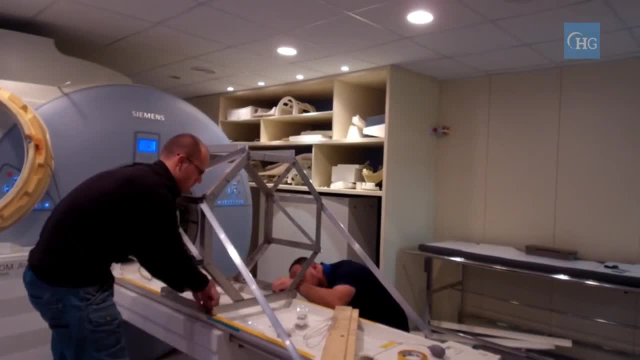 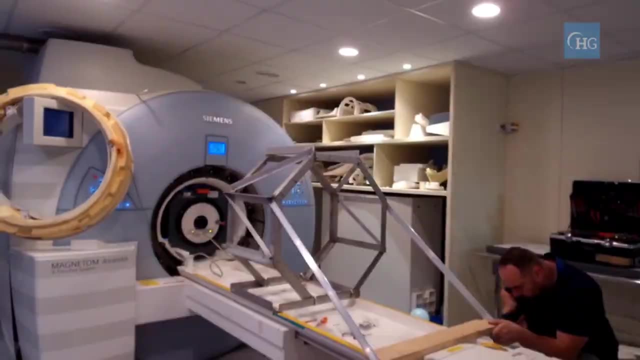 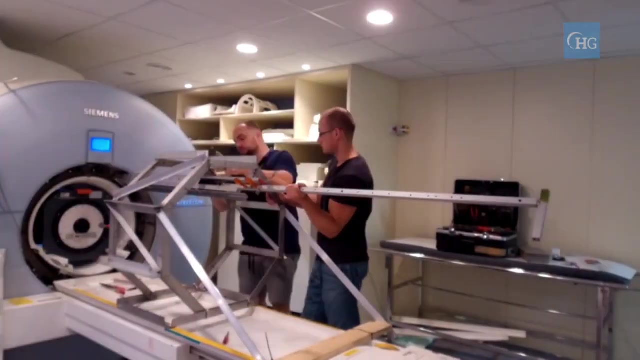 distortions in acquired images For humans or animals. the effect is particularly pronounced at air tissue boundaries, such as the sinuses, due to paramagnetic oxygen in the air, making, for example, the frontal lobes of the brain difficult to image. To restore field homogeneity: 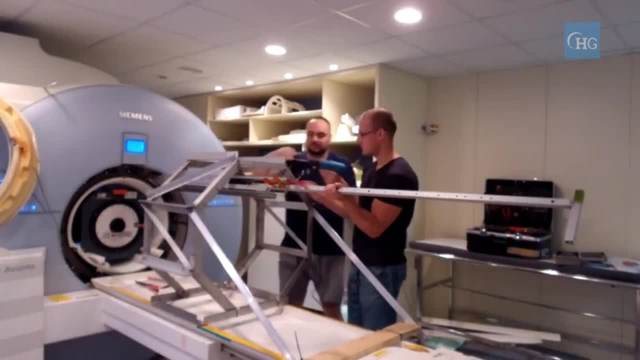 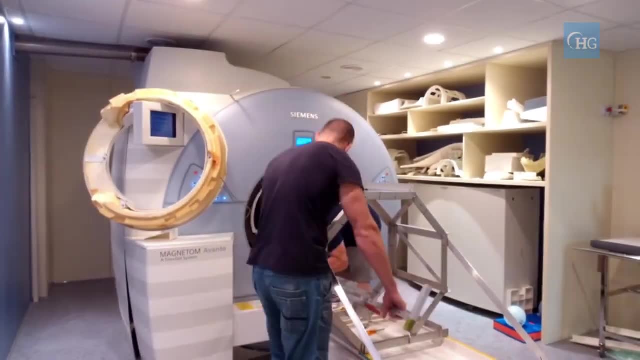 a set of shim coils is included in the scanner. These are resistive coils, usually at room temperature, capable of producing field corrections, distributed as several orders of harmonics. After placing the sample in the scanner, the field is shimmed by adjusting currents in the shim coils. 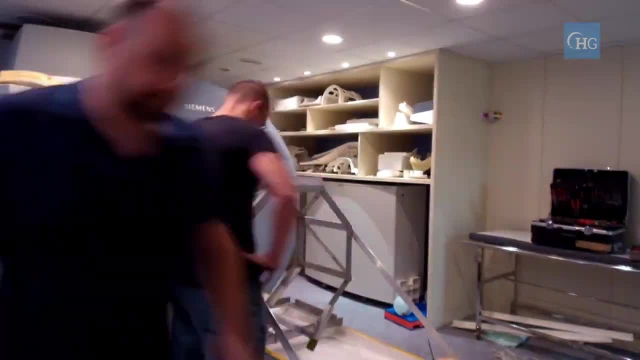 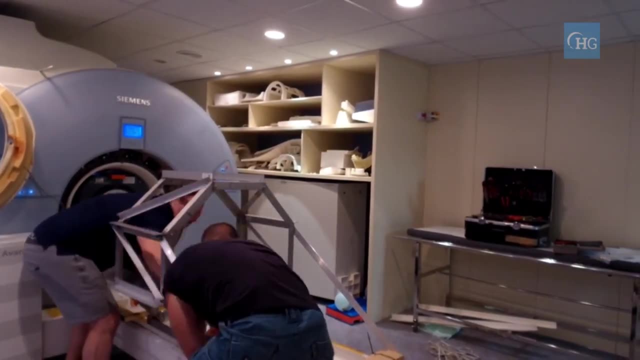 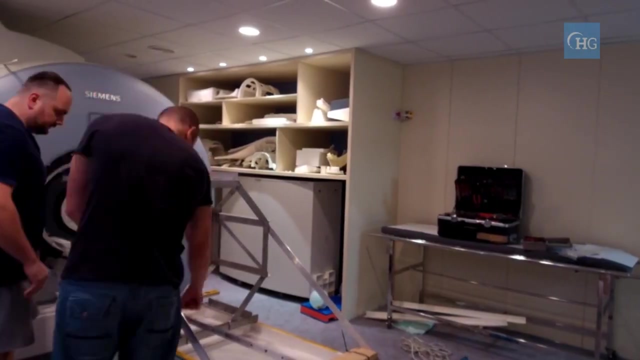 Field homogeneity is measured by examining an FID signal. in the absence of field gradients, The FID from a poorly shimmed sample will show a complex decay envelope, often with many humps. Shim currents are then adjusted to produce a large amplitude, exponentially decaying FID. 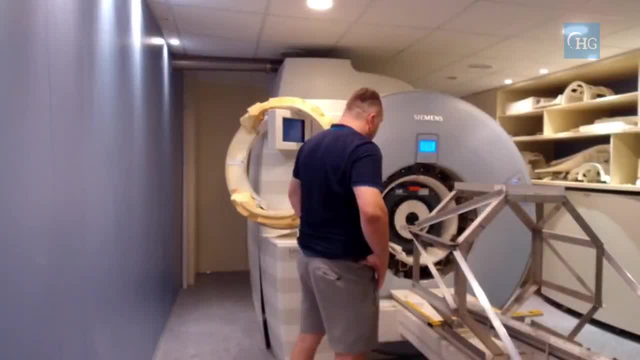 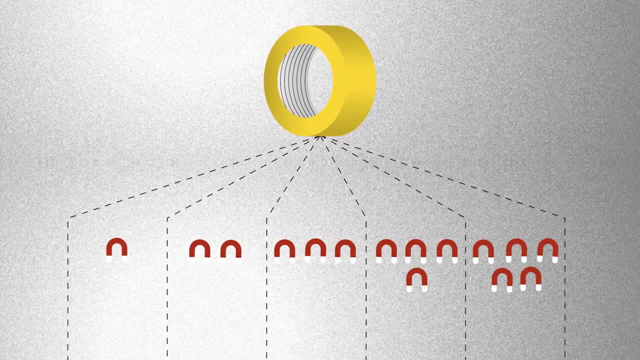 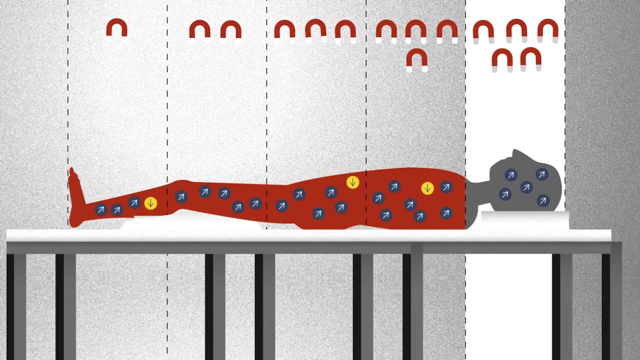 indicating a homogeneous field. The process is usually automated. The third component in MRI systems is the radio frequency system. The radio frequency or RF transmission system consists of an RF synthesizer, power amplifier and transmitting coil. The coil is usually built into the body of the scanner. 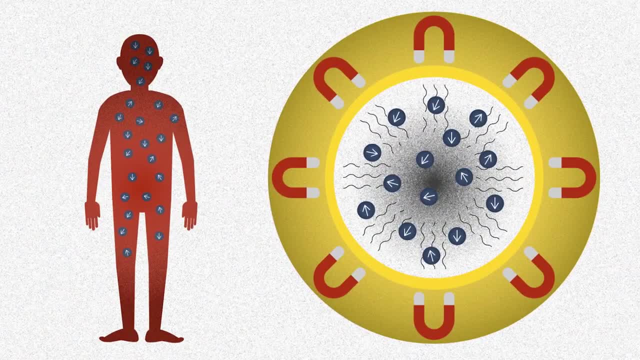 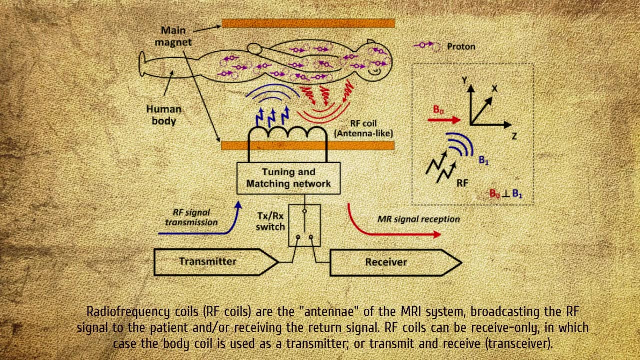 The power of the transmitter is variable, but high-end small-body scanners may have a peak output power of up to 35 kilowatts and be capable of sustaining average power of 1 kilowatt, Although these electromagnetic fields are in the RF range of 10s of MHz. 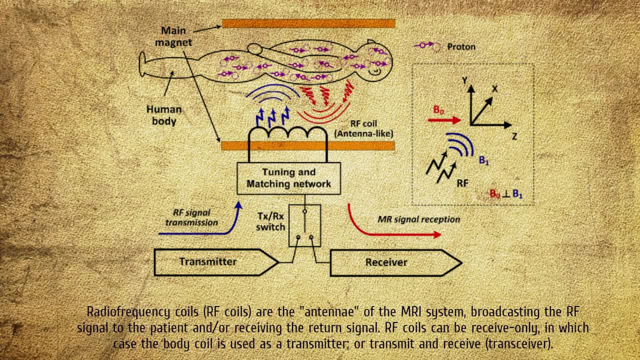 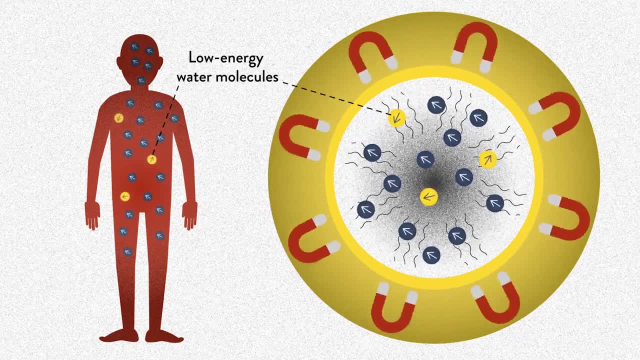 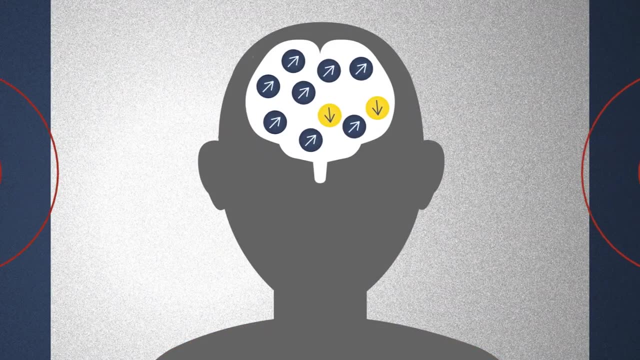 often in the short-wave radio portion of the electromagnetic spectrum at powers usually exceeding the highest powers used by amateur radio. there is very little RF interference produced by the MRI machine. The reason for this is that the MRI is not a radio transmitter. RF frequency electromagnetic field produced in the transmitting coil is a magnetic near-field. 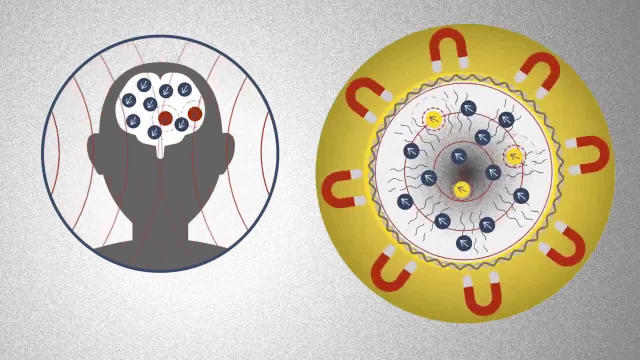 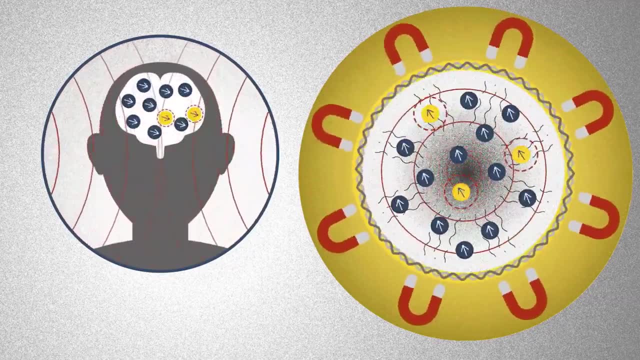 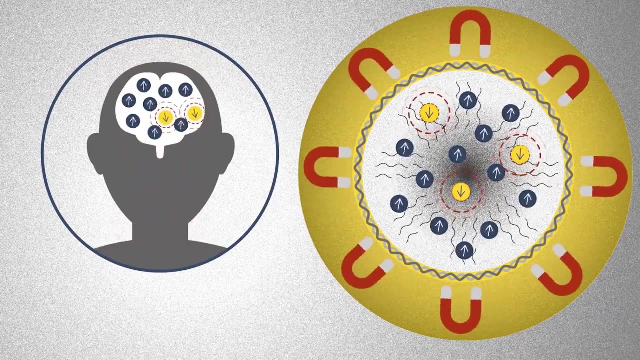 with very little associated changing electric field components, such as all conventional radio wave transmissions have Thus the high-powered electromagnetic field produced in the MRI transmitter. coil does not produce much electromagnetic radiation at its RF frequency and the power is confined to the coil space and not radiated as radio waves. 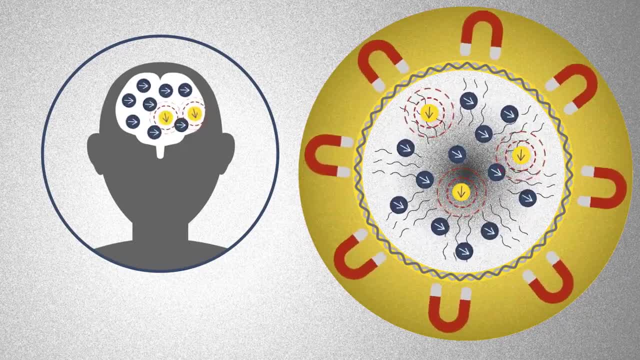 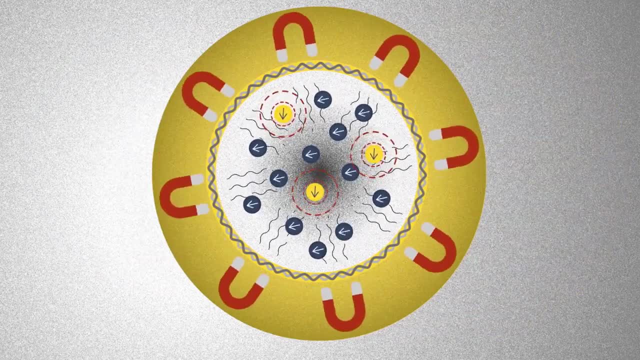 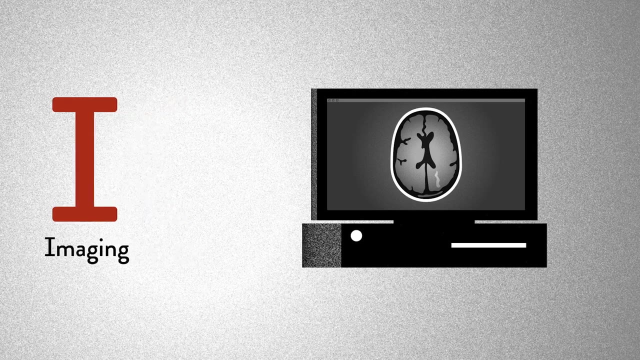 Thus, the transmitting coil is a good EM field transmitter at radio frequency, but a poor EM radiation transmitter at radio frequency. Let's look into different types of scans in the MRI system. There are a variety of different MRIs available. The most common MRIs include: 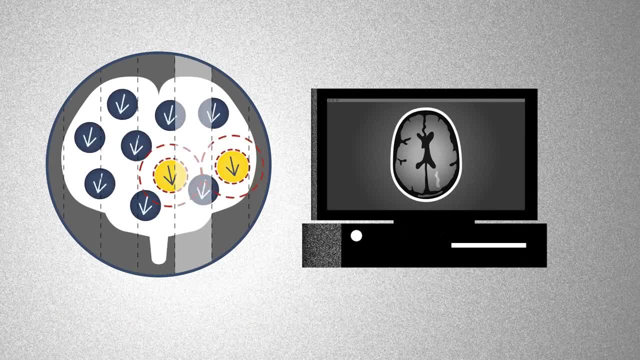 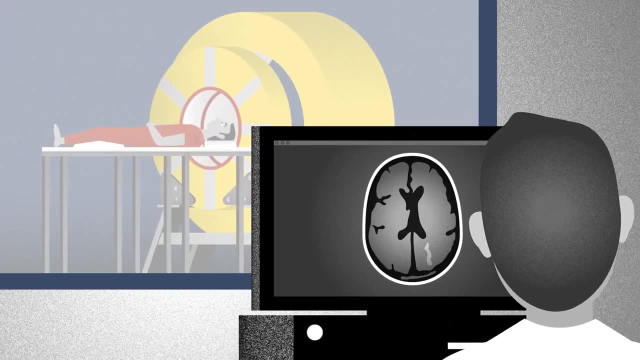 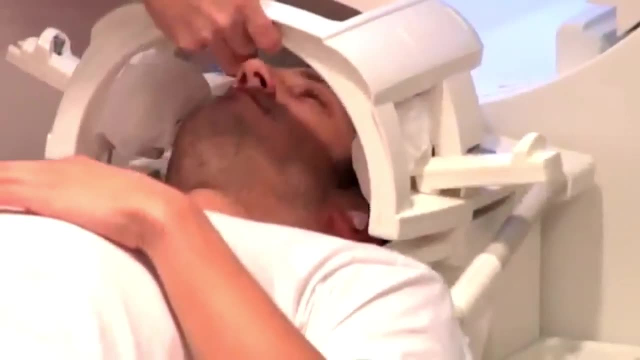 Functional MRI. A functional MRI or FMR tests brain activity. The images indicate whether there are any issues present that may predict or diagnose a stroke. A doctor also orders an FMR for brain mapping. Brain mapping is essential for brain surgery or for detecting epilepsy or tumors. Cardiac MRI. A cardiac MRI produces 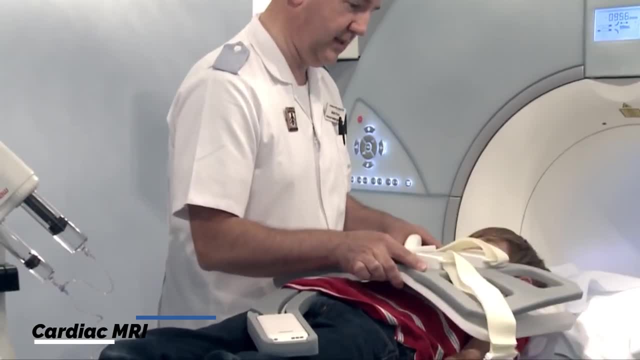 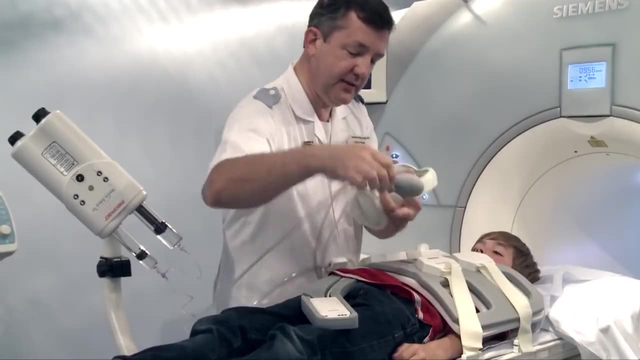 detailed images of the heart, Your doctor will call for a cardiac MRI to diagnose your condition so that a treatment plan can be devised. In addition to the heart, the blood vessels surrounding it are also examined. The information gathered is used to determine heart function. 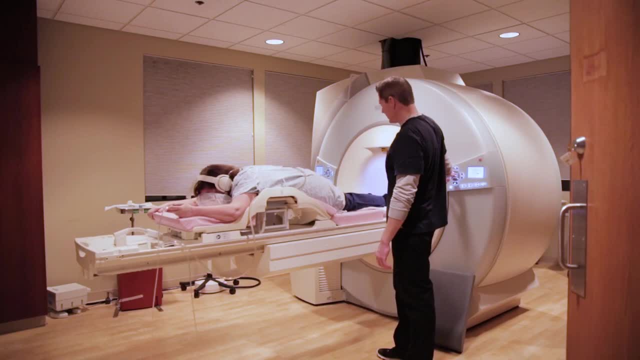 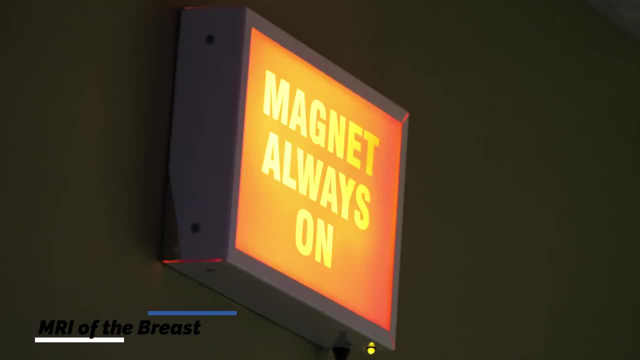 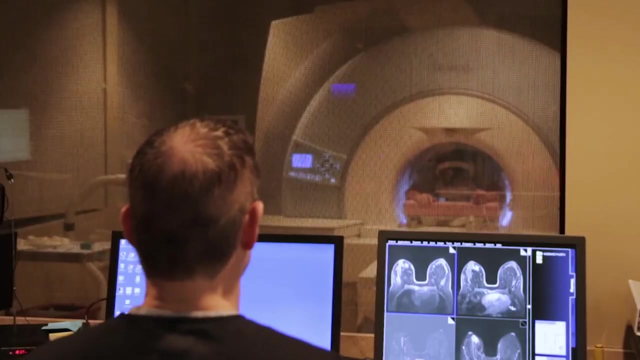 MRI of the breast. Patients who are at high risk for breast cancer are candidates for an MRI. While it is a non-invasive procedure, doctors may order an MRI-guided needle biopsy of the breast. The MRI will detect breast cancer and provide information on progression and location of the 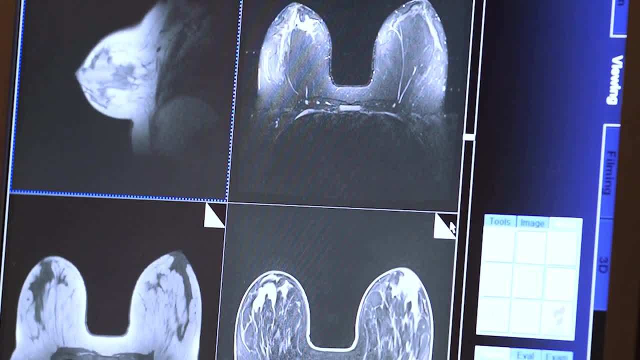 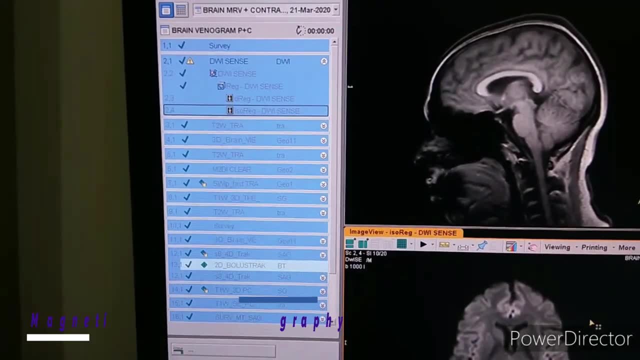 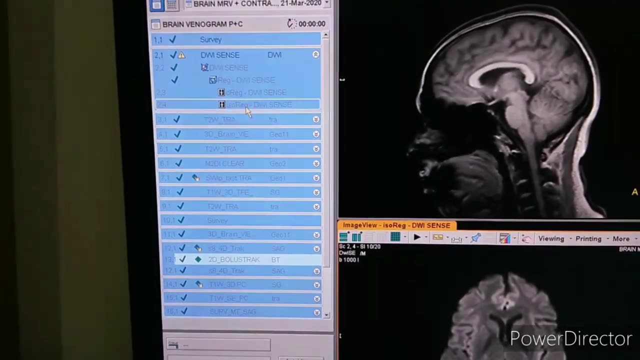 tumor. Magnetic resonance venography, or MRV, is combined with contrast dye to produce clear images of internal organs and other structures inside the body. The dye highlights the veins so that they appear translucent and show up well in the images. Magnetic resonance angiography is similar to an MRV. It combines images with an intravenous 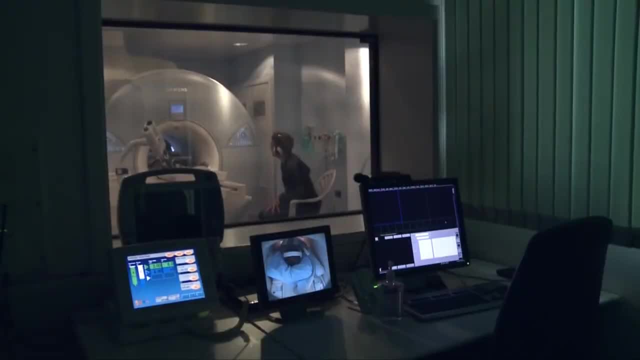 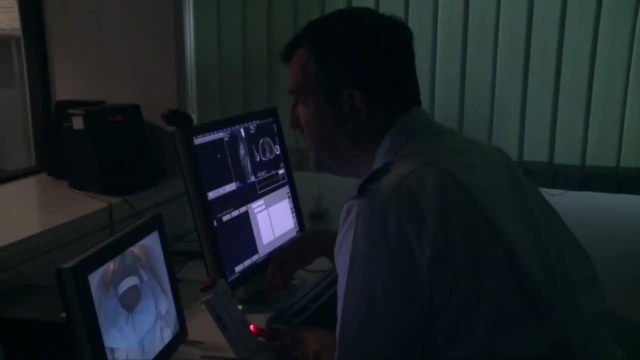 contrast dye but focuses on blood vessels instead of veins. The physician will be able to evaluate the blood vessels that run through the heart and soft tissues of the body. Non-contrast MRA. Some patients may be unable to tolerate contrast dye. This is especially 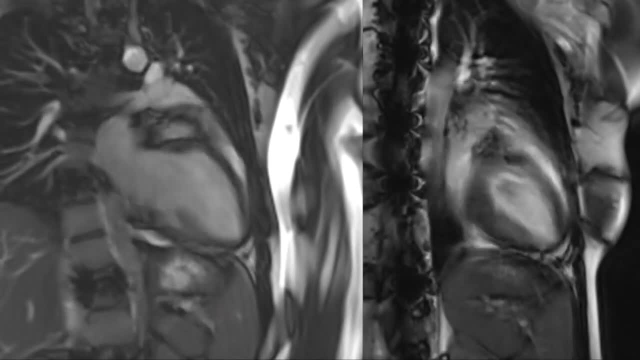 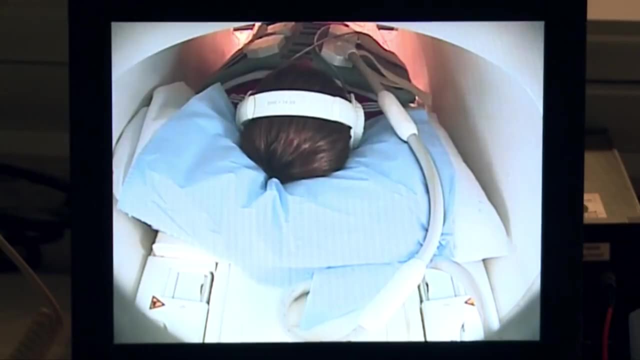 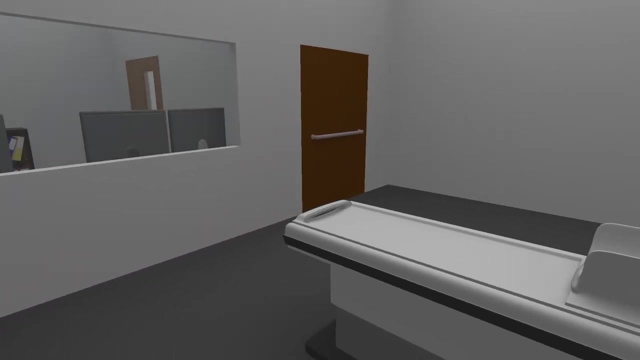 true for patients who have renal problems. Historically, these patients could not get MRAs performed. However, it is now possible for all patients to get MRAs using advanced diagnostic technologies that eliminate the need for dye, without compromising on clear images. Open high-field MRI Being closed in is a fear that some patients have in regards to an MRI exam. 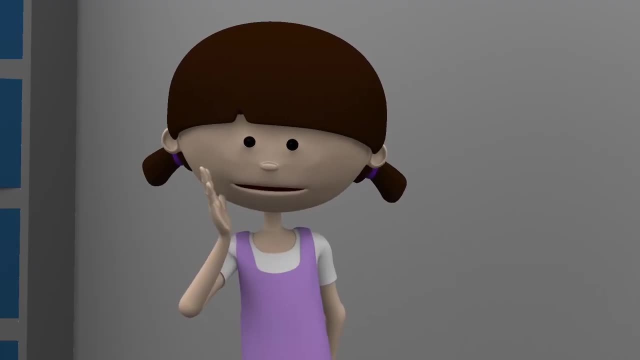 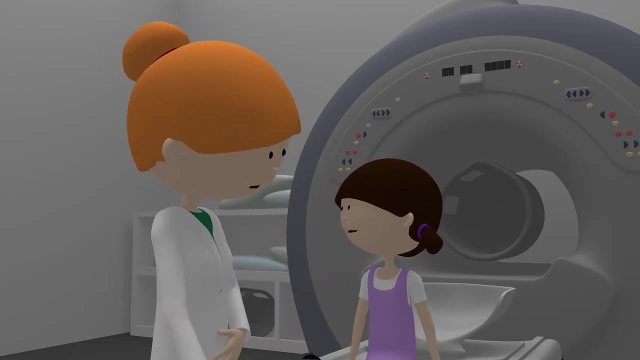 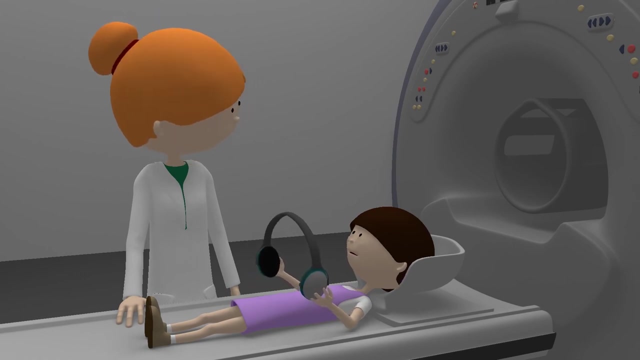 Patients who are claustrophobic don't like the design of an MRI machine that is enclosed. Other patients may be obese or suffer from post-traumatic stress syndrome, preventing them from feeling comfortable in the machine. For these patients, open, high-field MRIs are a better choice. Let's end this video with helium-less MRI machines. 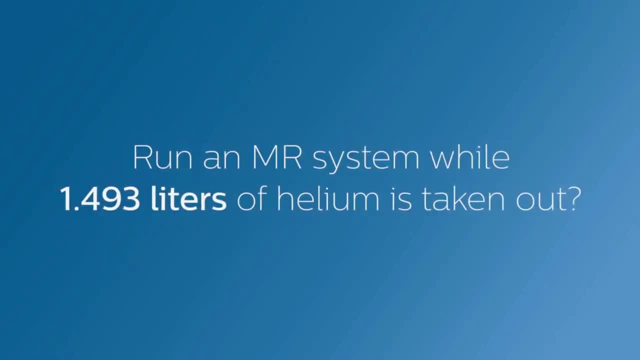 Critical in the use of high-field MRI scanners, which use helium to cool the superconducting magnets to 4 Kelvin or negative 269 centigrade. the declining of the high-field MRI is a major concern. The high availability of helium is causing waves of